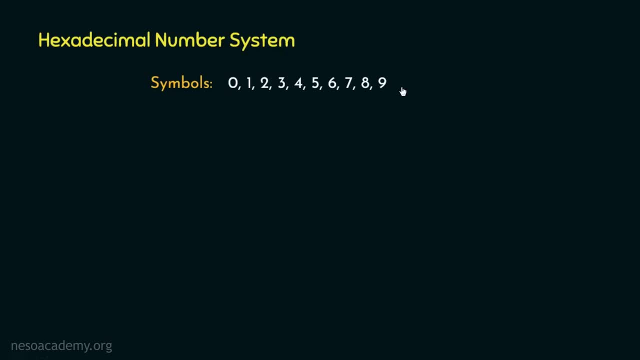 symbols are actually as same as the decimal number system, And in decimal we have these 10 symbols only. But here the situation is different. If we notice the name of this number system, it's hexadecimal. Now, decimal means 10 and this prefix hexa means 6.. So basically, 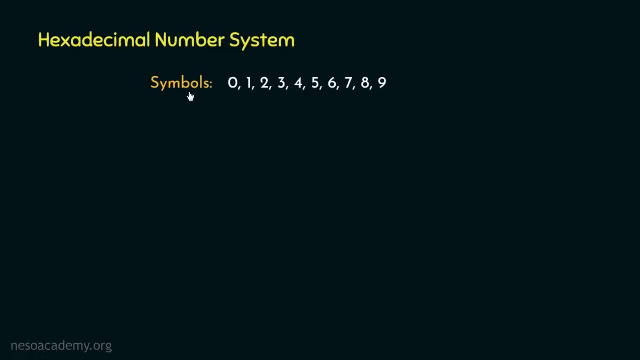 here we will have 10 plus 6, that is 16 symbols. Now, symbols of any number system have to be represented using a single element. In case of decimal number system, if you remember, after 9 we write 10.. That means the second symbol in line, that is, 1 in the 10th place. 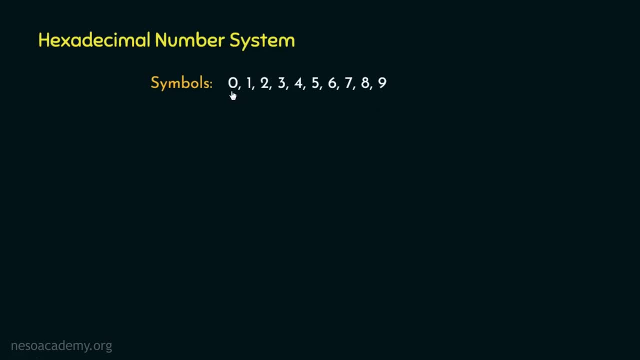 followed by the first symbol, that is, 0, in the unit's place. This happens because we have exhausted all the symbols in the unit's place by writing till 9.. Now, in case of hexadecimal, we are supposed to have 16 symbols, right? So we are yet to exhaust the symbols in the 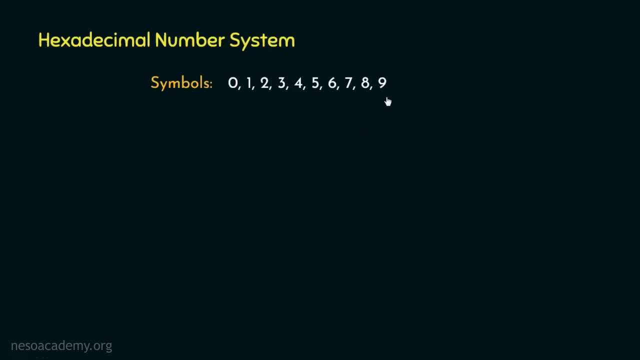 least significant digit's place. That's why, for representing the magnitudes after 9, we use the symbols like A, B, C, D, E and F. So in total here we have 16 symbols, and clearly that is the base of this number system. Now, similar to octal, hexadecimal also has a special 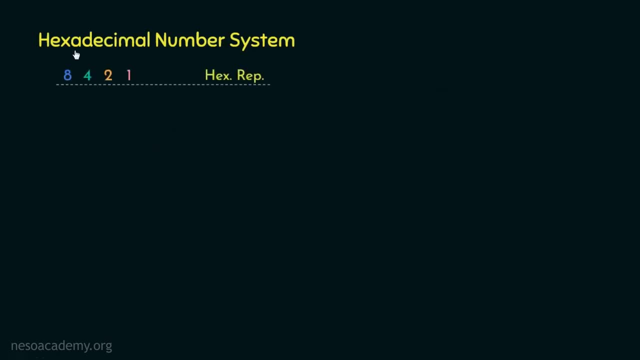 importance with the binary numbers. Basically, every 4 bit binary number represents a hexadecimal symbol. Let me illustrate Now. in case of a 4 bit binary number, the place values from the LSB to MSB are 1,, 2,, 4 and 8.. Well, this much we already know. right Now, 0000 in hexadecimal. 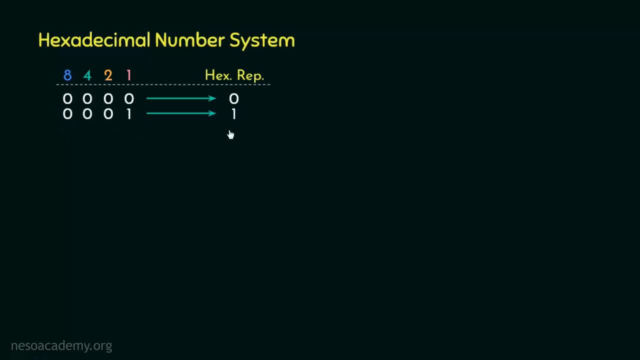 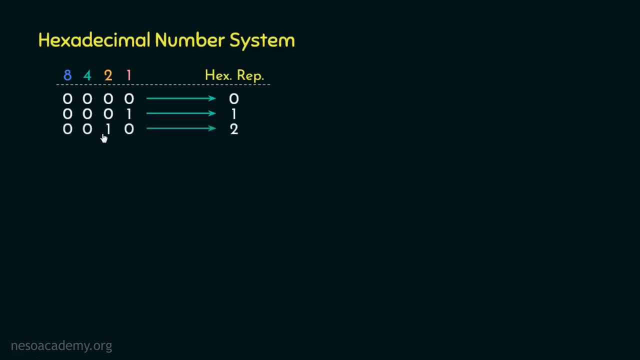 the ones placed underneath the place value: 1. 0010 is 2, as 1 is beneath 2.. 0011 is 3, because 2 plus 1 is 3.. 0100 is 4, as 1 is placed under 4.. 0101 is 5 because 4 plus 1 is 5.. Then 0110 is 6, because 4. 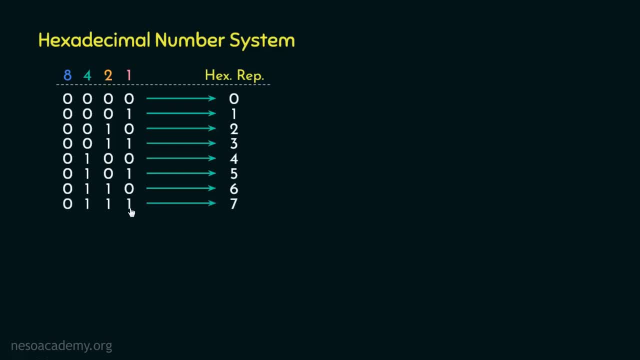 plus 2 is 6.. 0111 is 7 because 4 plus 2 is 6 and 6 plus 1 is 7.. Now 100 is 8, as 1 is placed beneath 8.. Then 1001 is 9, because 8 plus 1 is 9.. Now 1010 is actually 10 in decimal, because 8 plus 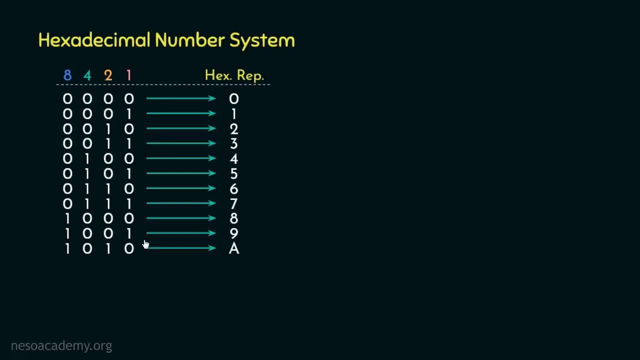 2 is 10.. But in case of hexadecimal we represent that magnitude using the symbol. Then 1011 in decimal would be 8 plus 2 plus 1, that is 11, which in hexadecimal is B. So 1100, that is 12. in hexadecimal is C: 1101, that is 13, in hexadecimal would be D: 1110, that is 14. 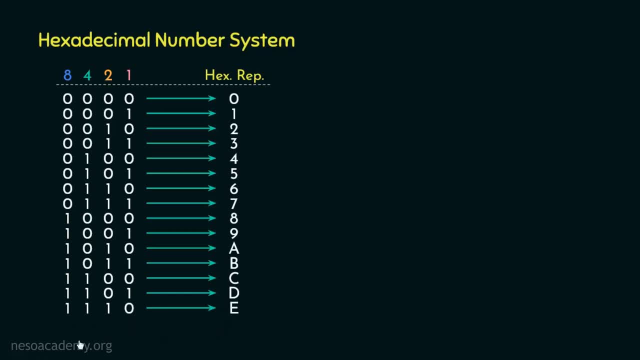 in hexadecimal would be E And finally 1111, that is 15, because 8 plus 4 is 12.. And 12 plus 2 is 14 and plus 1 is 15, which in hexadecimal is F. So these all are the symbols. 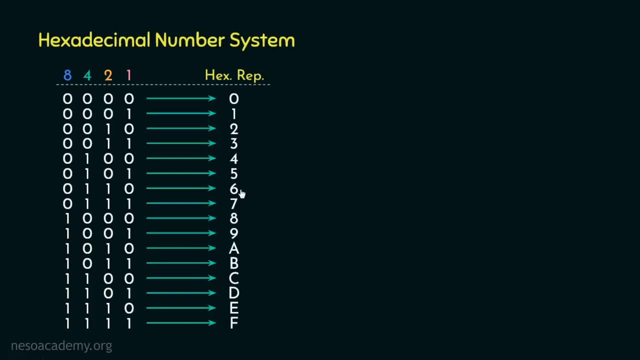 of the hexadecimal number system, Now similar to octal. this number system also comes very handy in the representation of binary bit streams using less than number of digits. Moreover, this number system has a greater impact due to its base. That means using this number system. 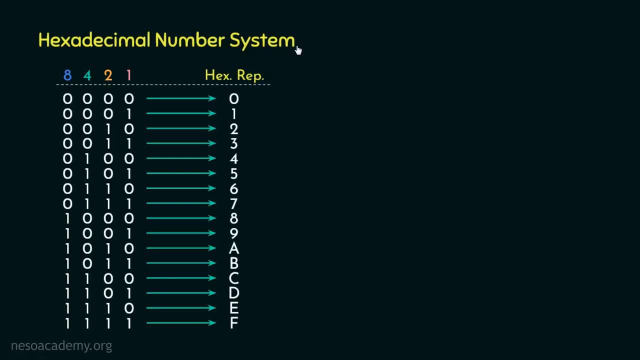 we can represent the number of digits, So this number system has a greater impact due to its base. That means, using this number system, we can represent the binary bit streams using even less than number of digits than octal. Consider this binary number Now in order to represent it. 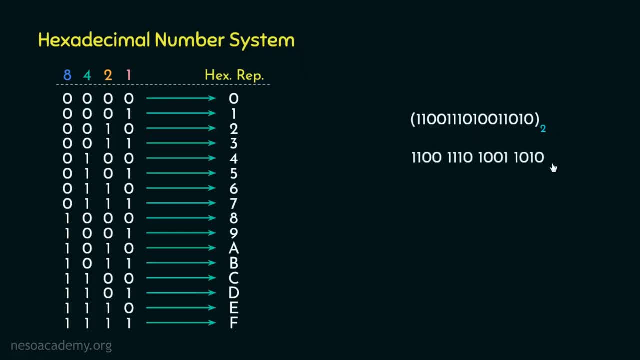 in hexadecimal, we will first make group of 4 bits from the LSB to the MSB. Now, since it was a 16-bit binary number, that's why these groups could be formed easily. In case the groups are not formed this smoothly, that is, after grouping 4 bits from LSB to MSB, if in the most significant group 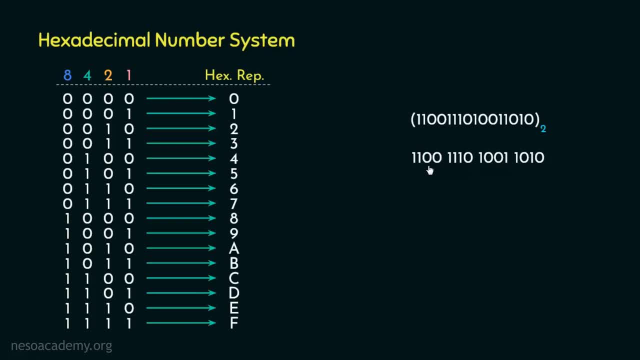 there are less than number of bits, then the number of digits could be formed easily. Now, in order to represent the number of bits, we can always append zeros to the most significant place, Because, except for unary, in all the other number systems we are free to append any number. 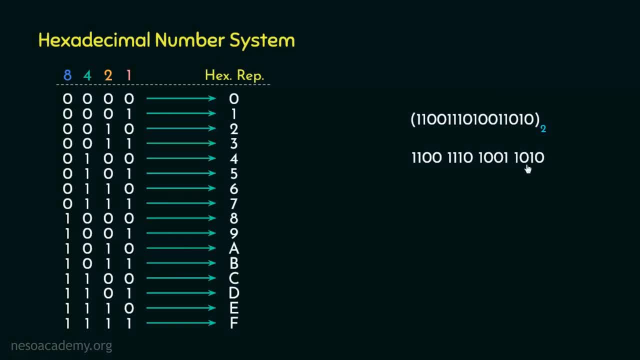 of zeros to the left of any number. Now 1010 in hexadecimal is A, then 1001 is 9,, then 1110 in decimal is 14, and in hexadecimal it is E, And finally 1100, there is 12 in decimal. 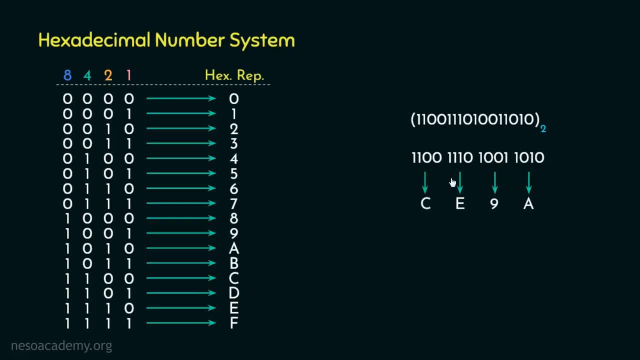 thencart, and then in hexadecimal is C. So the 16-bit binary number can be represented in hexadecimal with only 4 digits And the value of the binary number in hexadecimal is CE9A base 16.. Now hexadecimal numbers are also represented adding a prefix 0x in front of the number. 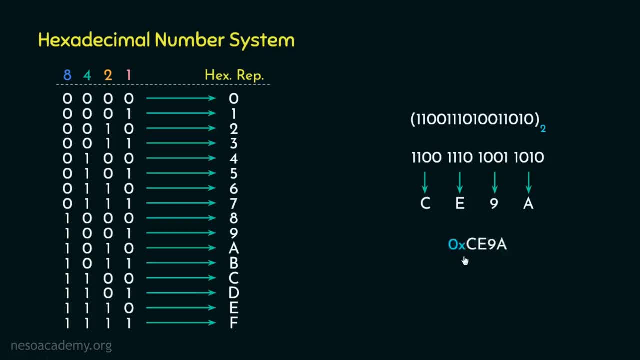 So this value can also be stated as 0xCE9A, Since using fewer hexadecimals, these examples are: bring out little bit Renee's number: måsteves Measure numbers using hex. planetary index is equal to min, 3x, min, 2x, min, 4x And number. 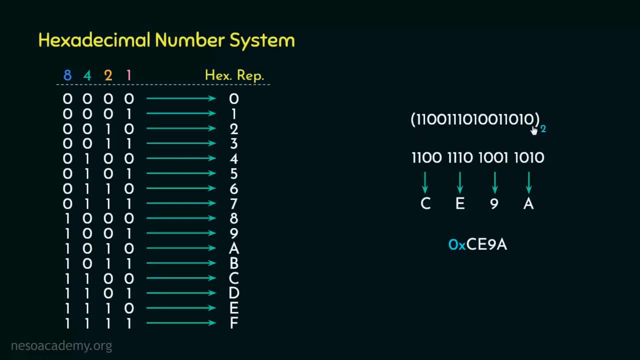 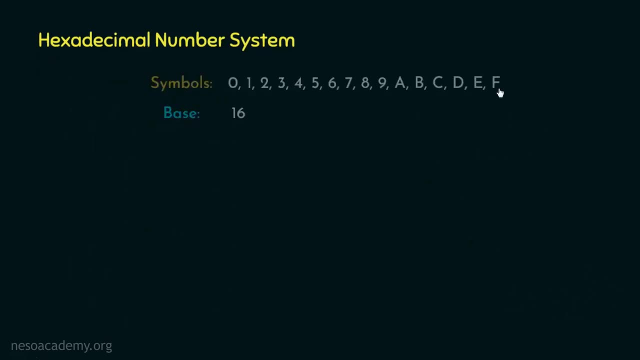 digits we can represent very long binary bit streams. Hexadecimal numbers are often used to represent the addresses in memory devices. Let's now observe how the numbers are formed in hexadecimal using these symbols, Now similar to the other number systems. first we will have all the 16. 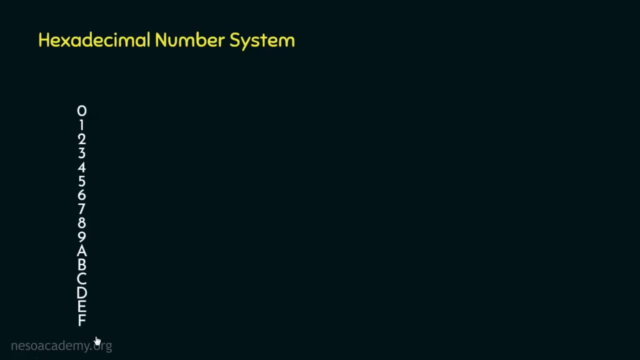 symbols. Now, after F, in order to form the next number, we will use the second symbol in line, that is, 1, in the most significant digits place and the subsequent numbers will be formed, placing all the 16 symbols in the least significant digits place, along with the symbol 1 as the most significant digit. 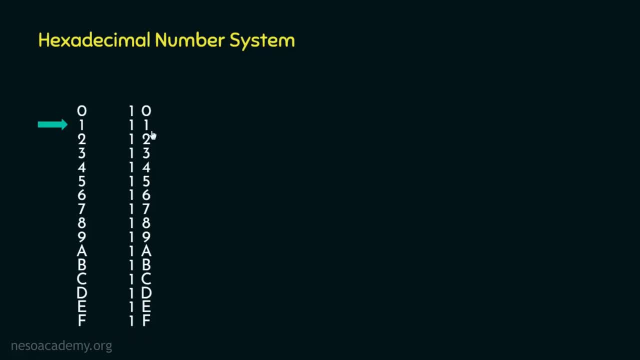 Since the least significant digit changes as the numbers progress, so naturally it will have the place value 16 raised to the power 0.. And observe, for 16 symbols in the least significant digits place we have 16 ones as the most significant digits place. Now let's see how the numbers are formed in hexadecimal. 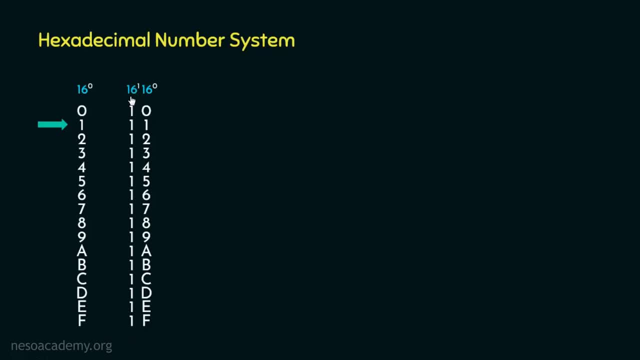 So it will have the place value of 16 raised to the power 1.. Now, eventually, for the most significant digit, we will reach 9, and for 9, once we use up all the symbols in the least significant digits place in order to form the next number. 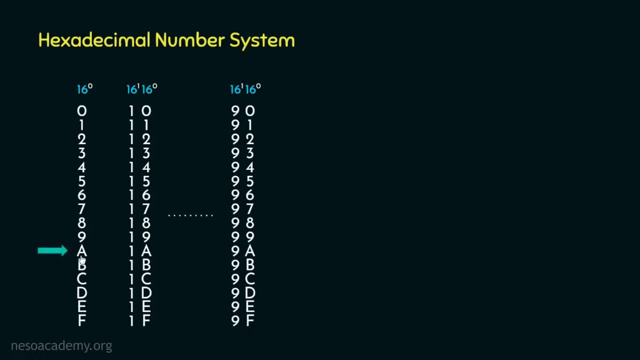 after 9 F, we will select the symbol A for the 16 raised to the power 1's place and perform the same drill. So the numbers after 9 F will be A0, A1, A2 till AF. Now, after AF, we will select the next symbol, that is, B for the 16 raised to the 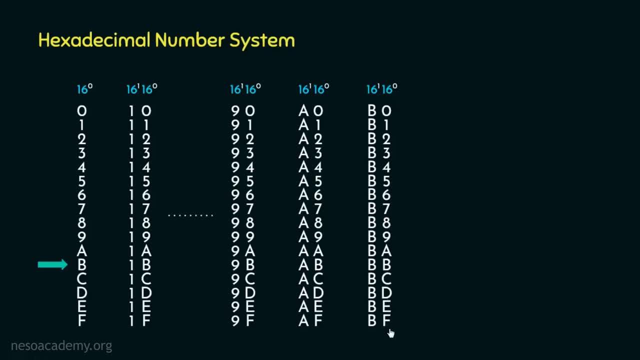 power 1's place, and 16 new numbers will be formed, with B as the most significant digit. Thus, there will come a time when we will reach F for the 16 raised to the power 1's place, and 16 new numbers will be. 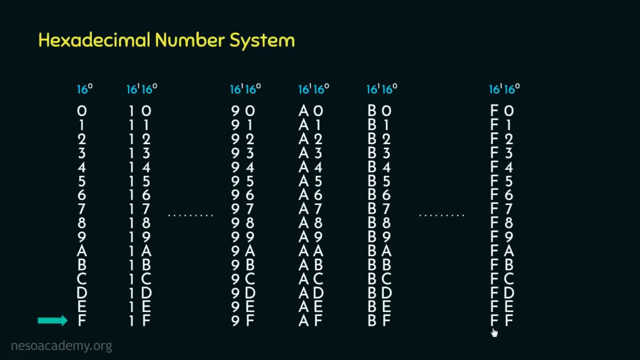 formed, having F as the most significant digit. At this point we have exhausted all the symbols that we have in these two places, So in order to form the next number, we will have to introduce a new place having the place value of 16 squared, because these two places are already exhausted. So, after FF, the next. 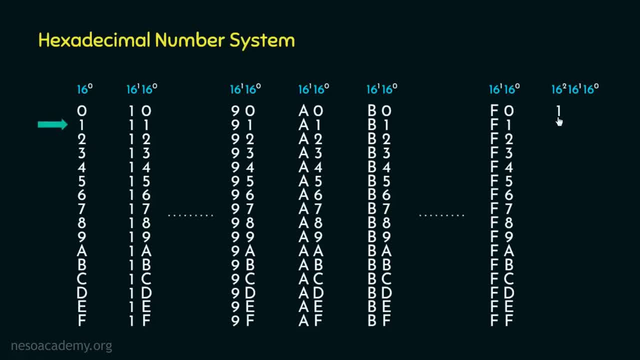 number will be formed by placing the symbol 1 in the 16 squared place And simultaneously these two places will be reset to 0's. So this is pretty much how the hexadecimal number system works. Now, before moving ahead, I have a question for you: What comes before and after the hexadecimal number CE9A? 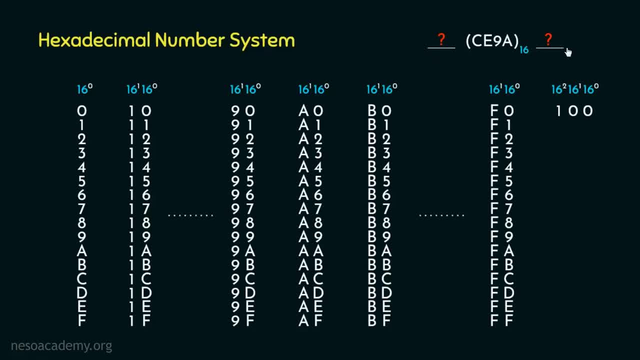 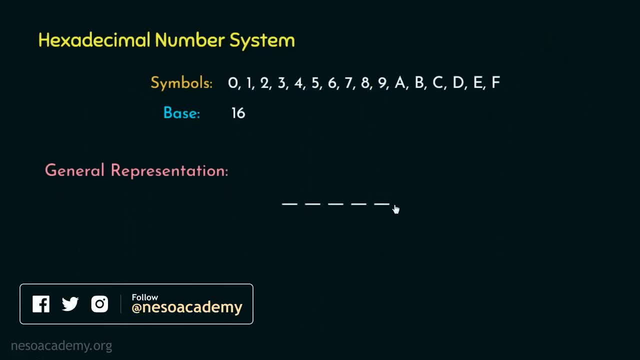 Feel free to write down your answers in the comment section. Now, coming to the general representation, consider a five-digit hexadecimal number. Now, all these places can have any symbols from 0 to F and, being a hexadecimal number, it will have the base as 16.. Therefore, the place values will be. 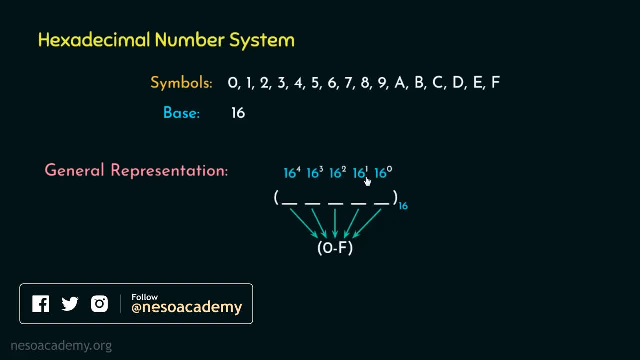 16 raised to the power 0,, 16 raised to the power 1, 16 squared, 16 cubed till 16 raised to the power 4.. Because although it's a five-digit number, the place value of the least significant digit began from 16 raised to the power 0. So for the